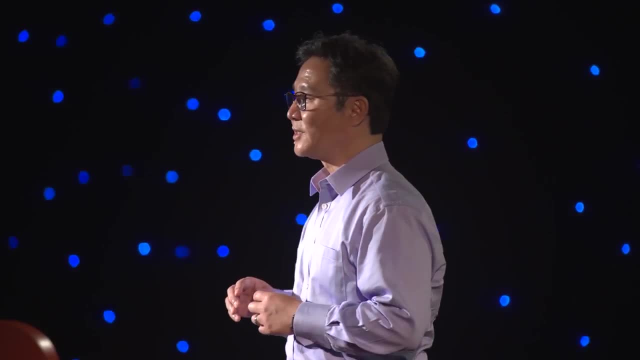 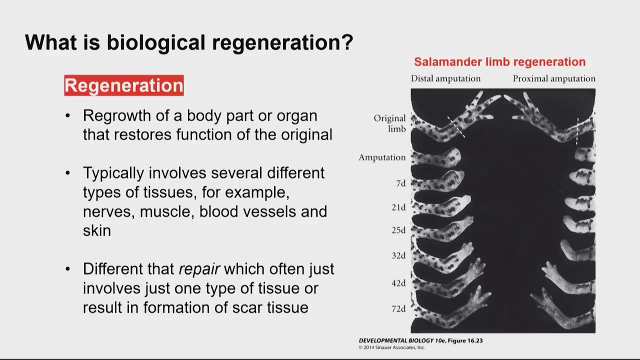 things, And on the right side you'll see a pinnacle of example of regeneration. So salamanders can lose their forelimbs or their hind limbs and then they actually can grow back at almost nearly identical replacement, truly regenerating what was lost, You know. 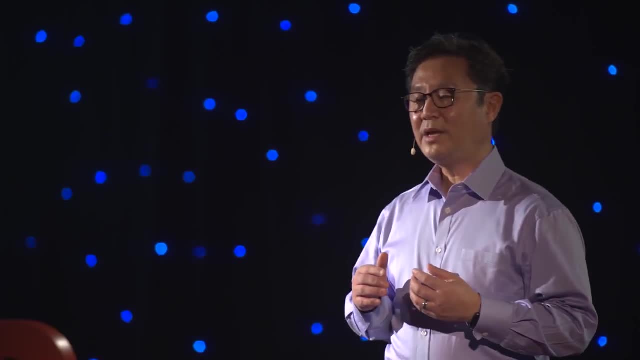 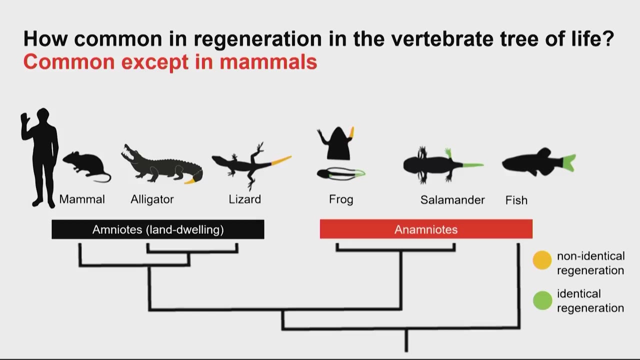 you could ask yourself: so how common is this, Dr? So we are, you know, part of a group of animals that have backbones, called vertebrates, And you could see, like how common is regeneration in the vertebrate tree of life? And the answer is actually it's. 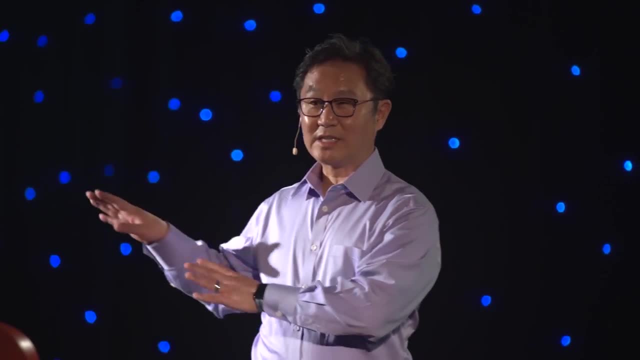 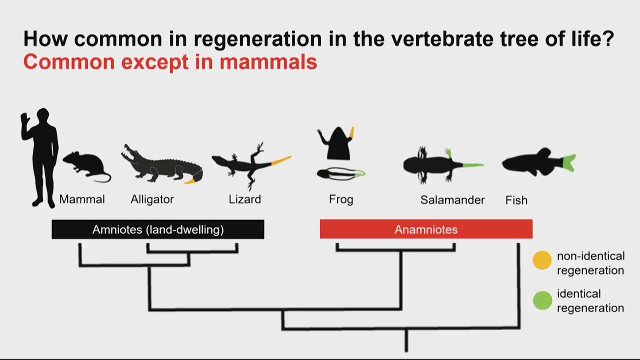 pretty common. So let's start from a more distantly related. you know members of the vertebrates, So that group of animals is called anamniotes and they primarily live in the water. So examples are like the salamander we just saw and also a fish, And they actually 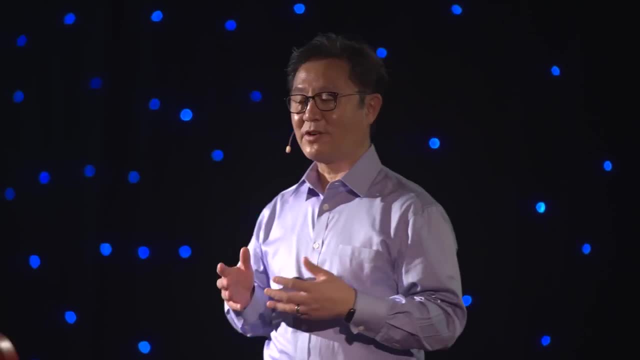 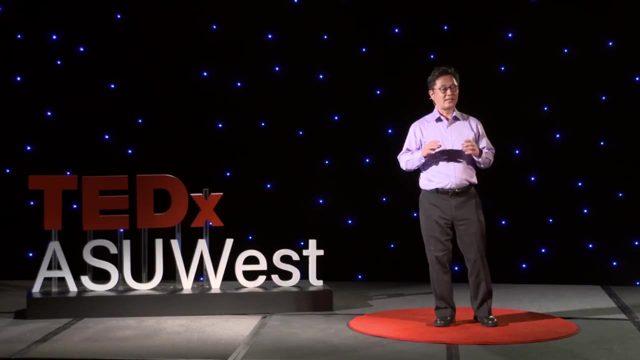 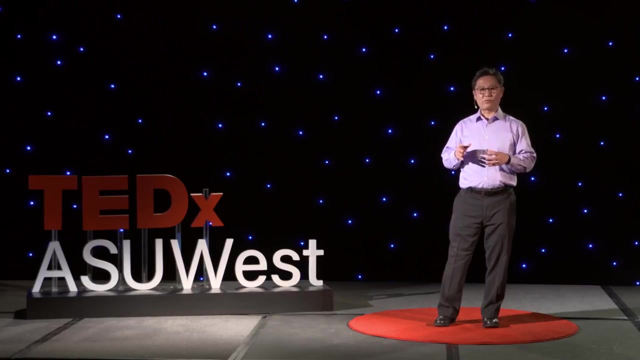 can exhibit something called identicals or perfect regeneration, So the part is pretty much exactly what was lost. In frogs you see something a little bit more complicated, where as younger animals they can regrow pretty much exactly identical regeneration, But in adults they actually don't recreate the part exactly. So it's. 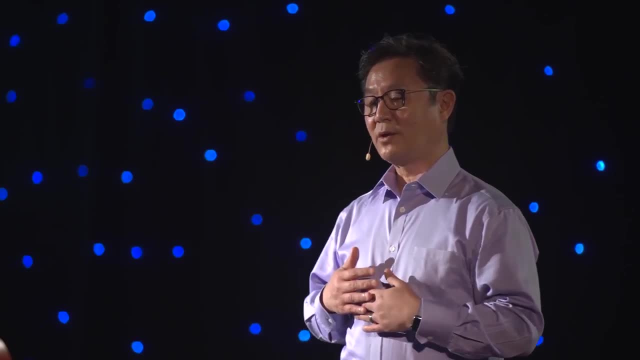 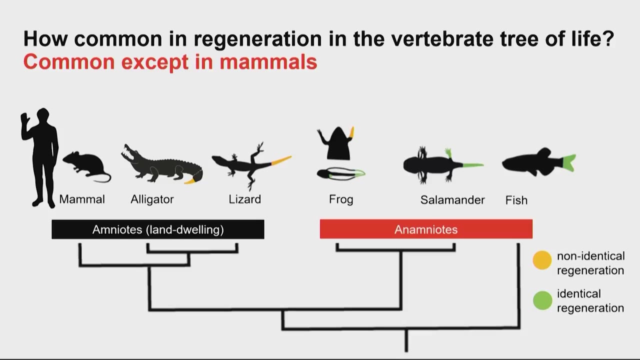 non-identical regeneration. Now, the group of animals that we belong to in vertebrates are called the amniotes, And the amniotes have evolved to live on land, And when we look at amniotes that can regenerate like reptiles, like alligators and lizards, that 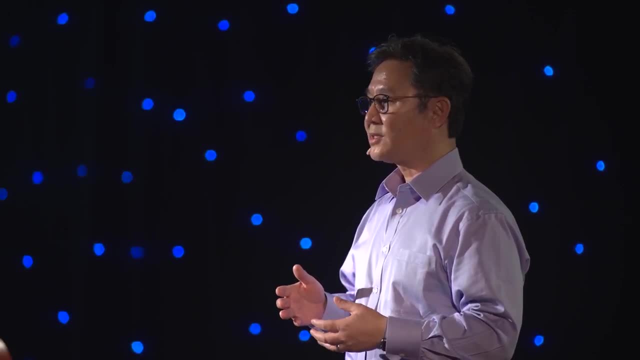 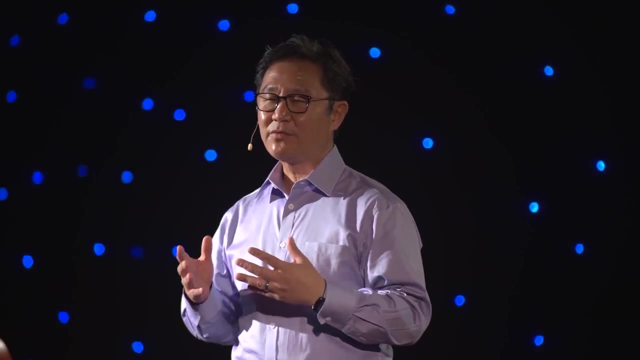 have lived, they are able to carry out non-identical regeneration. So the parts that regrow replace what was lost, but they're not exactly the same. So you know, that gives us a bit of a window into what might be happening, or capable of happening, in us as humans. So 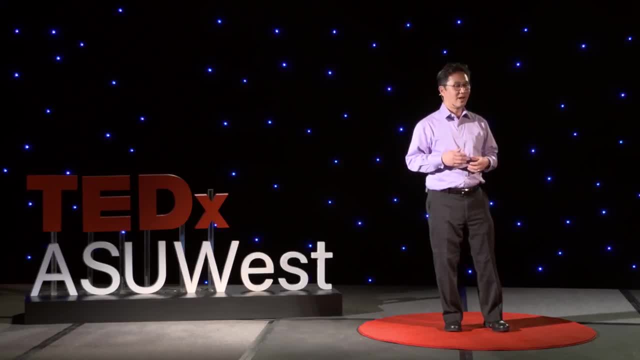 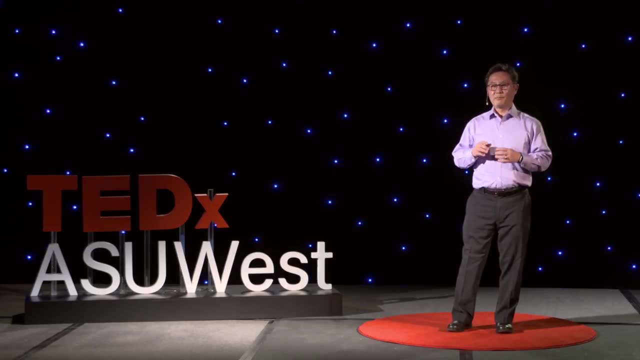 we are, you know, a member of an amniotes called mammals, And so mammals, we got the short end of the stick and we actually are not very good at regenerating. We have very limited ability, But because all of our vertebrate tree-of-life cousins can regenerate, we can. 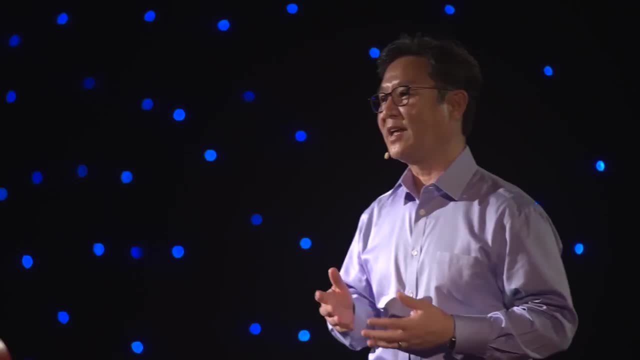 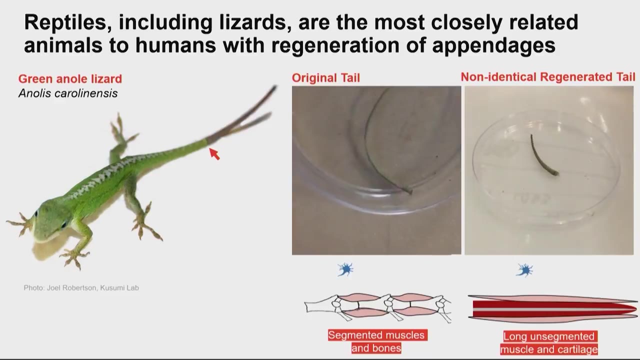 do that, You know. that actually raises hope about what can we, you know, reactivate in us. So what can we find out looking at reptiles and what they can do, Because they actually are the most closely related vertebrates to us that actually regenerate really well. So 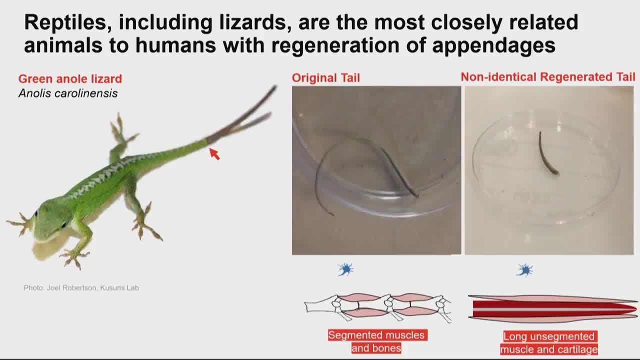 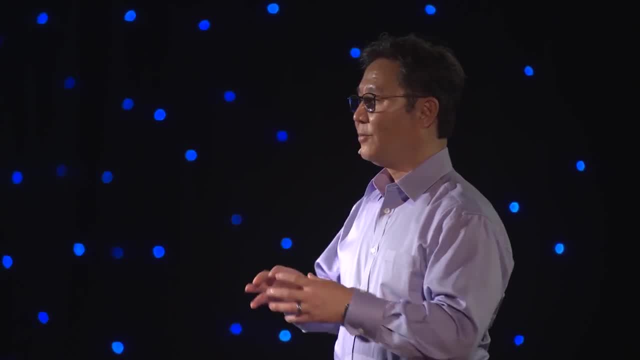 we've been doing studies on the green animal lizard on the left And we chose that because it has a whole genome, a whole set of genetic instructions that have been decoded, So we can look at that entire genetic sort of book of life and figure out which ones are the. 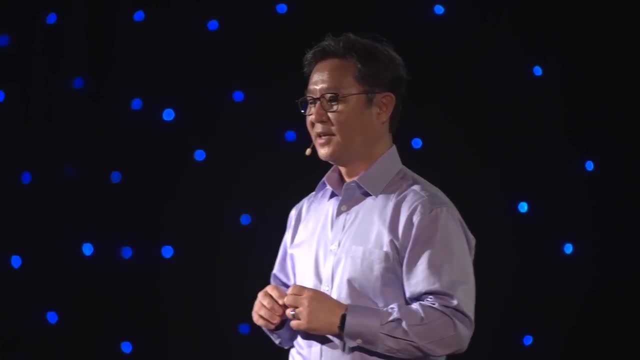 most likely reptile. So we finally have a set of genetic instructions that have been decoded, So we can look at that entire genetic sort of book of life and figure out- you know, okay, well, what might be involved. And then the- you know, lizards are able to lose their 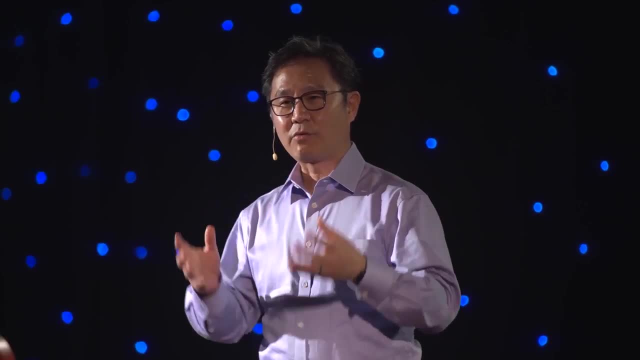 original tail and then you know that regrows and you can see, you know why. so they've evolved ability to lose their tail. What's good about that? Well, it wiggles, it distracts the predator. 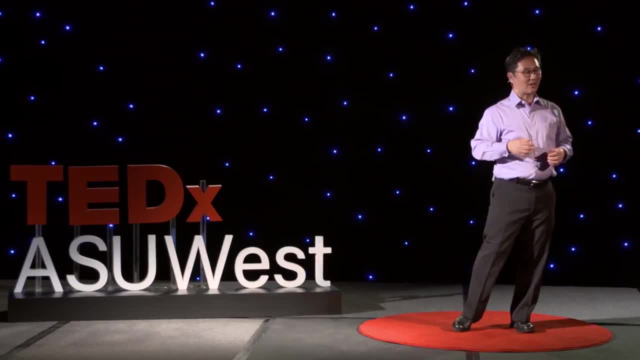 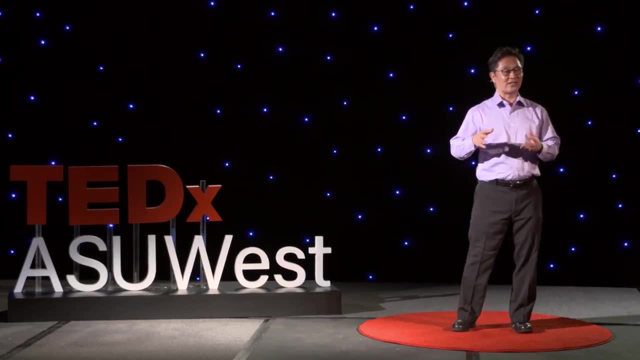 like your cats may have like, tried to grab a tail. The lizard, you know, runs off and survives to another day. But interestingly, the regenerated tail can also wiggle and it does replace that function of distracting the predator. Now what's interesting is that the original tail is 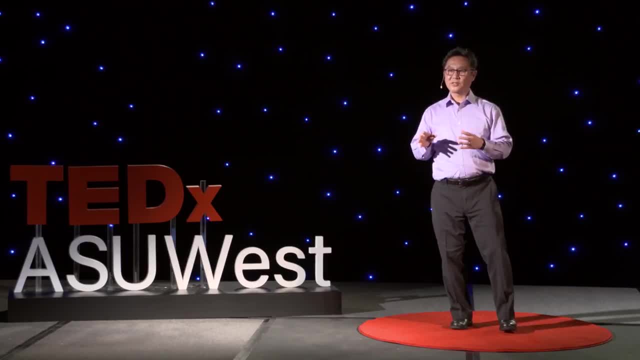 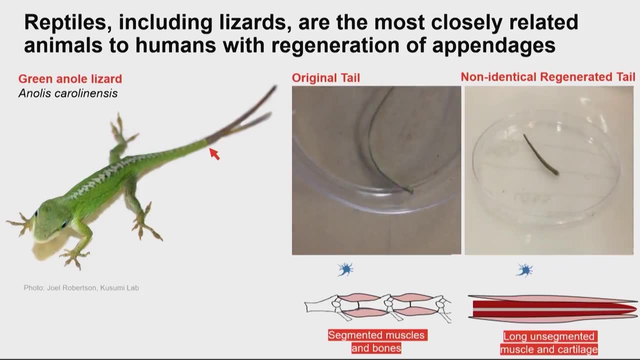 structured very differently than the regenerated tail. The original tail consists of segments of bone and cartilage and muscles, nerves, and you know it has actually slightly different motion. if you look at it, It's more sort of S-shaped or snake-like- The regenerated tail actually. 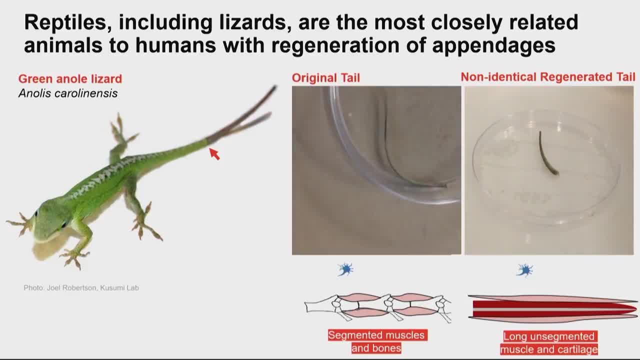 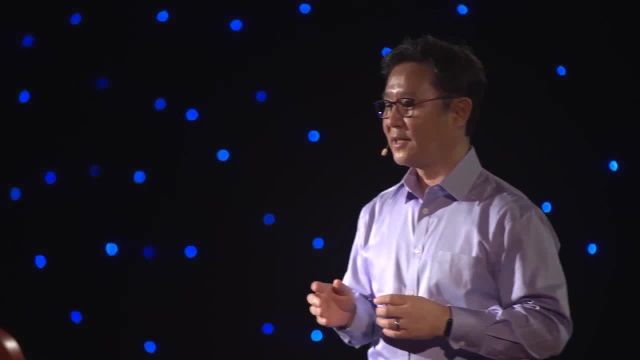 consists of just one long section of a cartilage, you know a cartilage tube that then is bent by these long muscles. So on the outside it looks pretty similar, but on the inside it's actually a good example of non-identical regeneration. So what we've done is been taken. 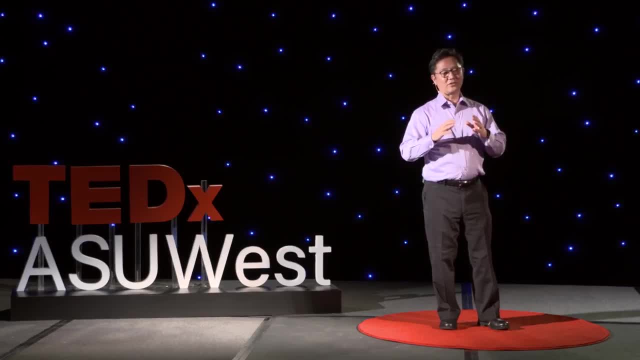 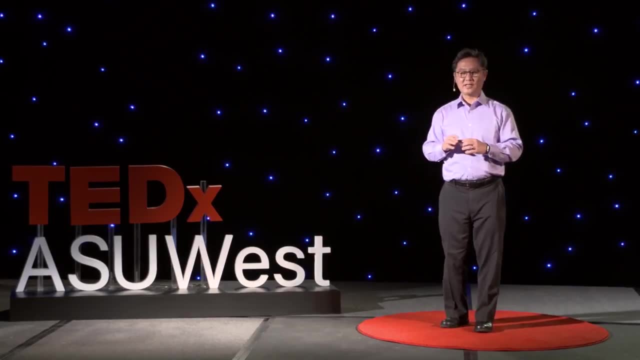 advantage of the fact that we have all the genes you know decoded in these lizards to look both at different stages in this process and also in different places in the regenerating tail. And what strikes us is that there are certain patterns that you see when you look at all 20,000. 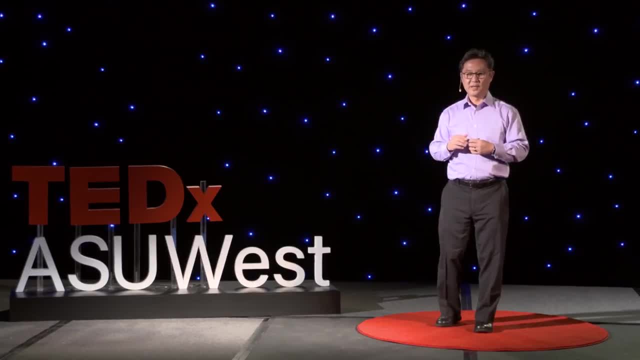 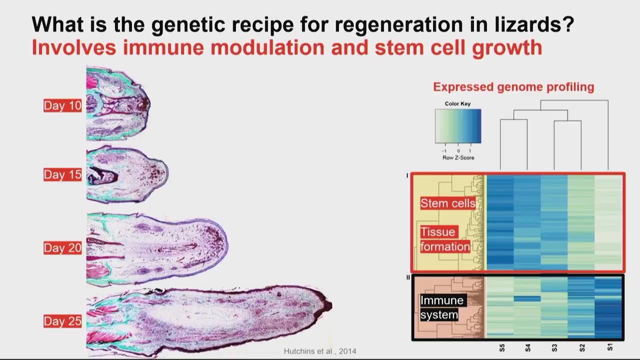 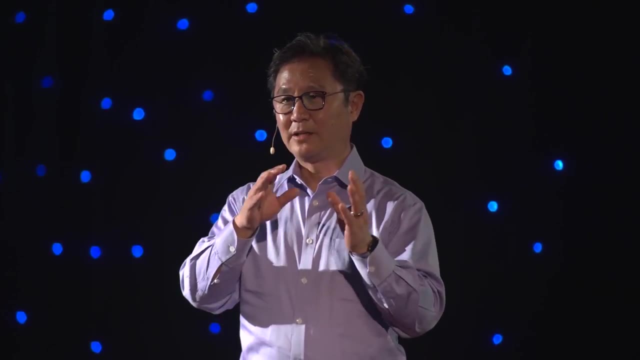 of the genes that are found in the lizard genome. So one class of cells that a class of genes that we find are those involved in stem cells. So these are cells that are capable of making multiple different types of tissues as well as reforming tissues, And we saw that particularly a little bit later. 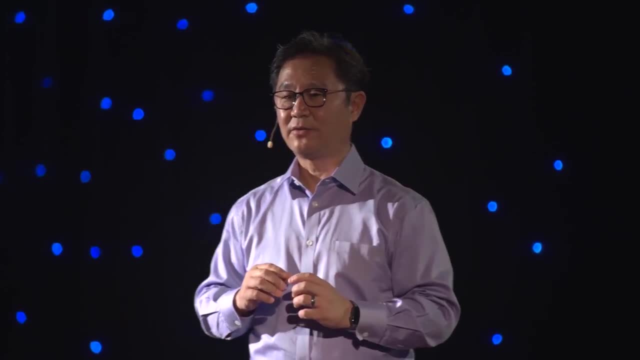 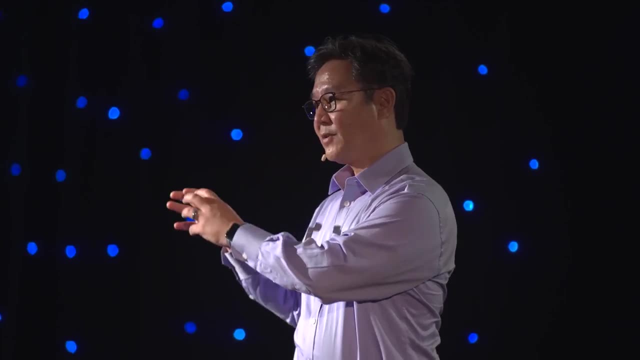 in regeneration and especially towards the base of this regenerating tail- The other group actually we saw very early, really early in the process of regeneration- and actually also towards the tip of the growing tail, And those are genes that control the immune system And that actually is. 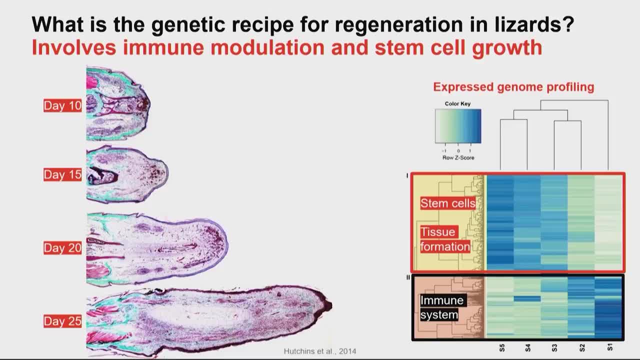 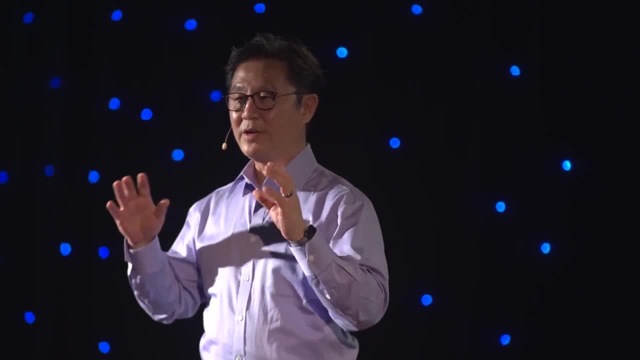 going to be really important for what I'll talk to you about next. And then this overview basically kind of is the one of the first of three. I think parts about what will be involved in the recipe to reactivate regeneration, or activate regeneration in humans. 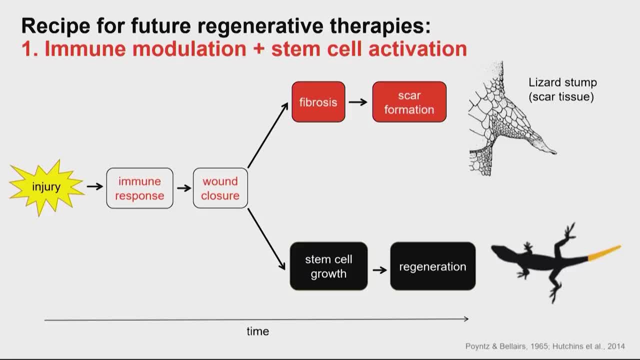 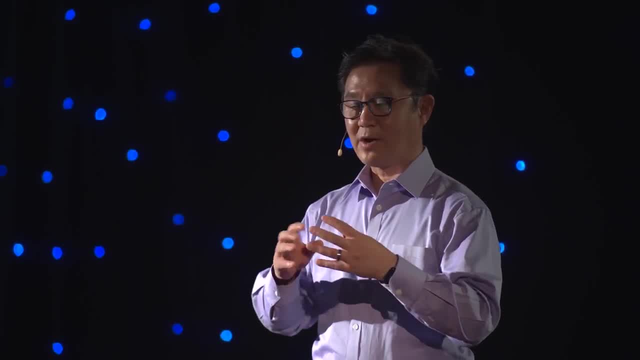 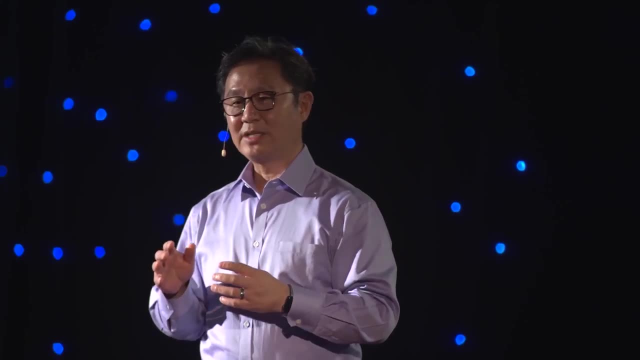 So regeneration is a response to injury. I mean, we've heard there's all kinds of injuries that we suffer, but then pretty soon on, there's an immune response. Either it gets red and hot and inflamed or it doesn't. And that immune response for, say, if you lose a limb or a tail. 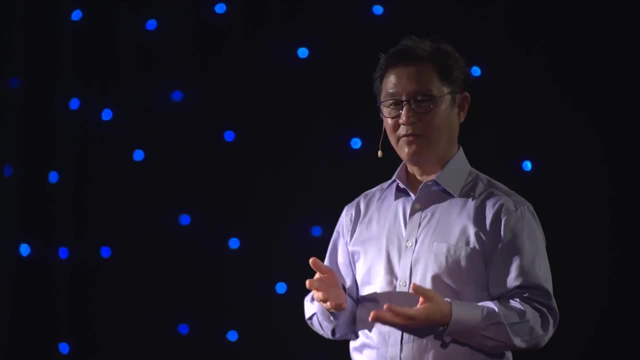 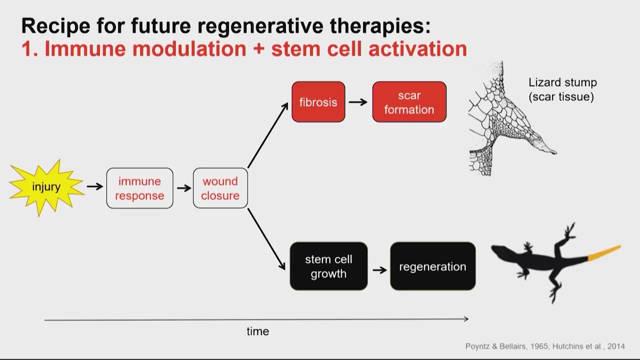 you need to close that up and close up the wound because you might get infected. And then, if you do set off certain kinds of reactions like inflammation, you start a process called fibrosis and that leads to scars And I think we all have scars in our body And the scars 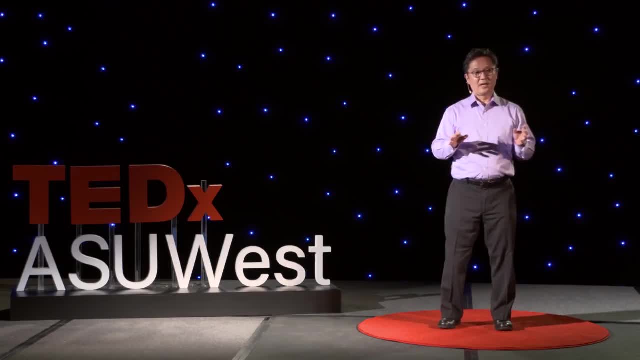 aren't as good as the original tissue, but it's better than having an open wound. Or if you have a heart attack and this muscle turns into scar tissue, it doesn't, you know, beat and contract like the original muscle, but it still prevents then a hole opening up in your heart. So and 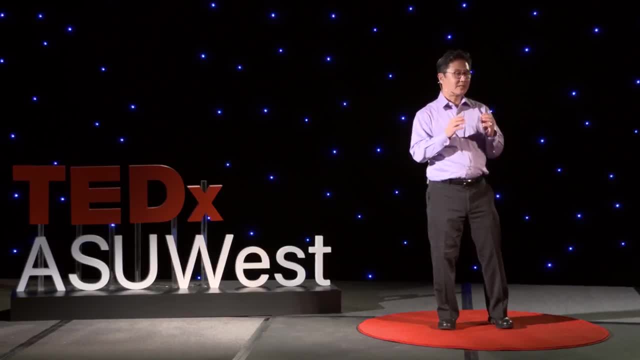 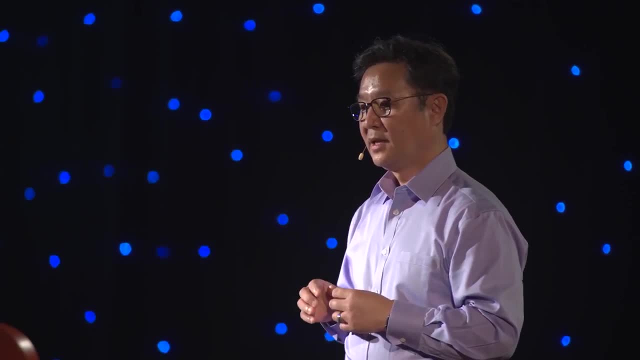 actually in lizards. actually, if you they lose a limb, what happens is it looks like it's starting to try to regrow, but then it pretty much immediately again goes into becoming a scar tissue. So if you have the right kind of immune response that you sort of suppress that scarring, 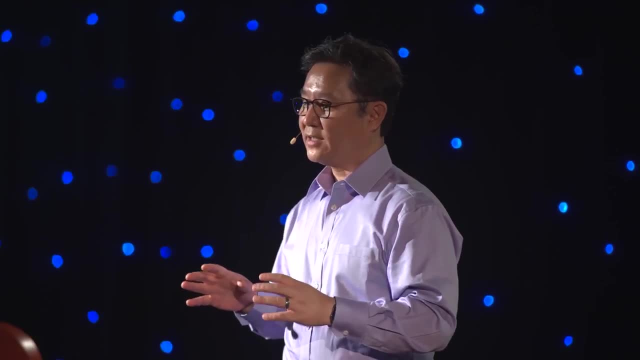 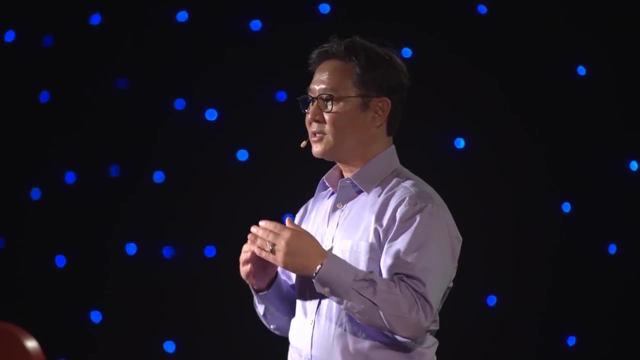 process and you allow those stem cells to get reactivated and, you know, lead the process of regeneration, then you can actually then get truly get a replacement of that part. So this kind of decision about which path on this tree that you go down, 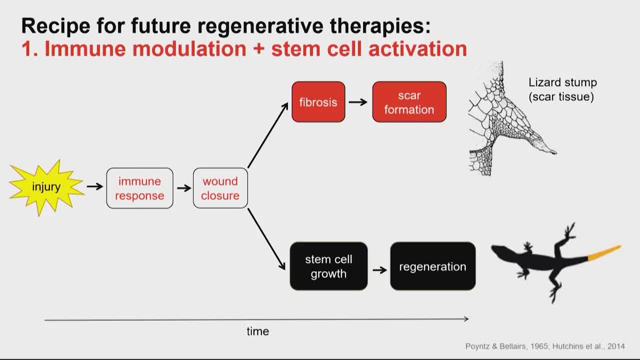 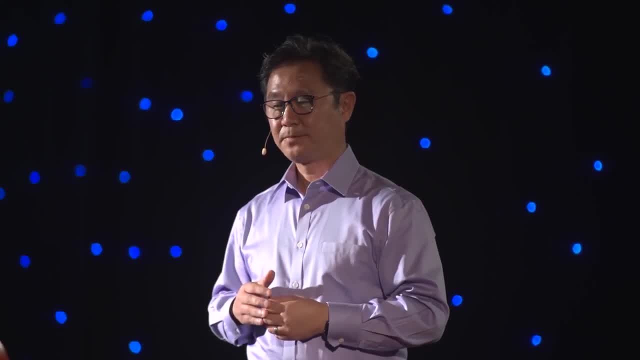 is really critical and really decided by the immune system. So what happens early on in the post-injury period makes a big difference of what might happen to the process next. So the second part- I think that is clear from studies that we've done- is that regeneration. 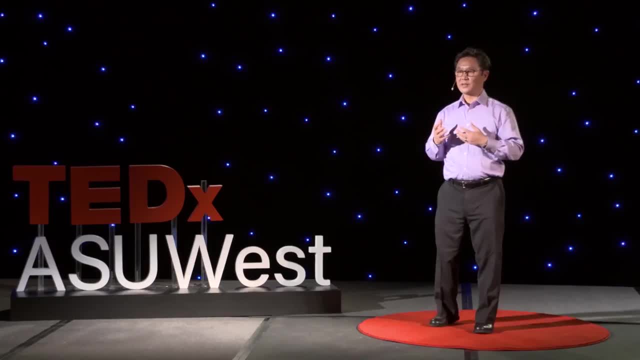 you know, is you know there's a reason why we as mammals, don't regenerate as well. So we looked at a certain type of stem cell that in us, in mammals, make muscle. So if you go to the gym and work out, you know, these cells, you know, help the muscle to bulk up. 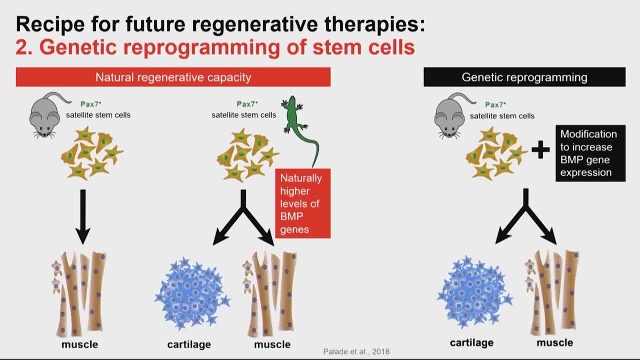 they're called satellite cells and they express certain genes on their surface. So normally if you take those out and you put them in a Petri dish and you culture them, they can make muscle. Now what's interesting? that if you go to the lizard and look for exactly the 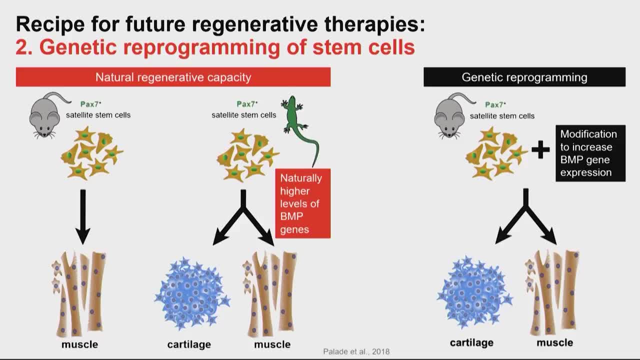 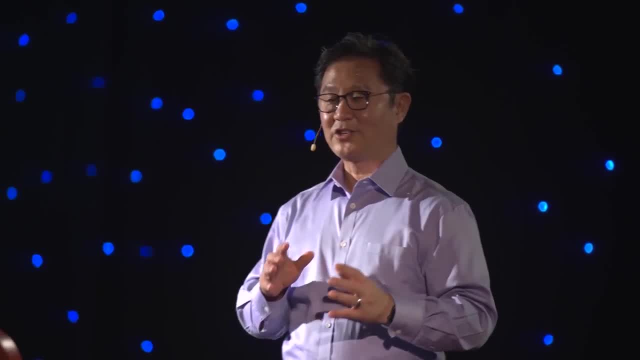 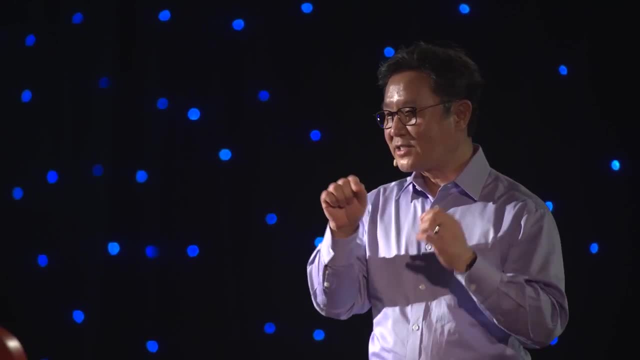 same kinds of cells that look exactly the same and express the same things. on their surfaces. they actually not only make muscle, which is kind of what you would expect, but they actually make cartilage too. And that's surprising because in us, you know, our satellite cells can't make cartilage. and when you go and look at what genes are on in 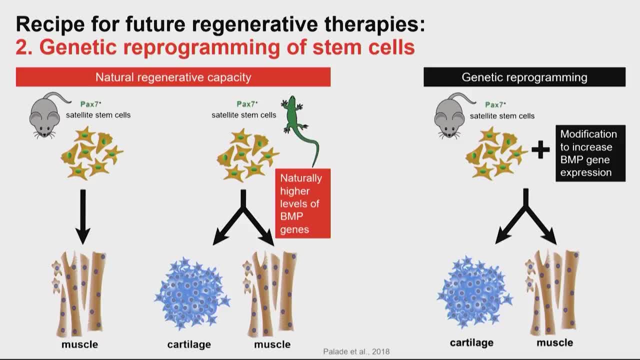 these cells. what it looks like is they're particularly really high levels of a gene family called BMPs, and BMPs really are important in activating cartilage formation. so essentially the lizards are already sort of naturally primed to make both muscle and cartilage, so we're not 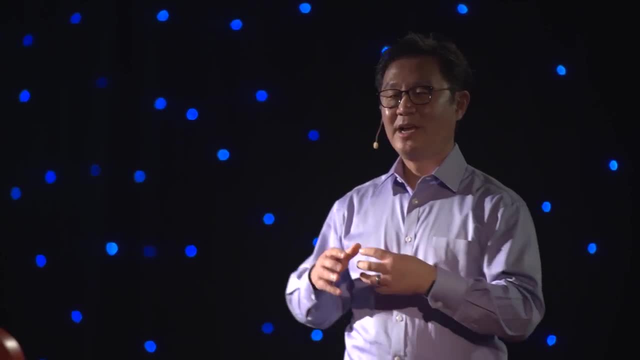 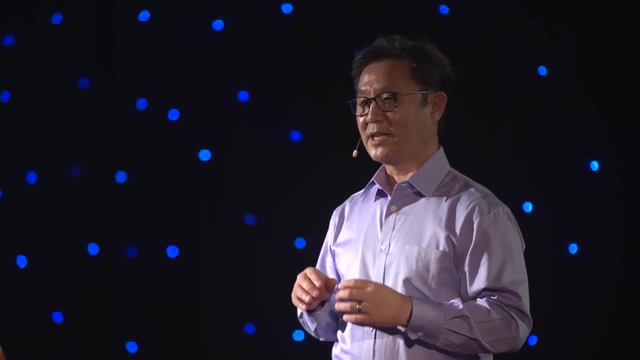 naturally primed to make muscle and cartilage. so if we wanted our cells- for example, for these satellite cells- to be more flexible and more capable, we would need to take advantage of genetic engineering technologies that exist, now that we can take cells, reprogram them, and they 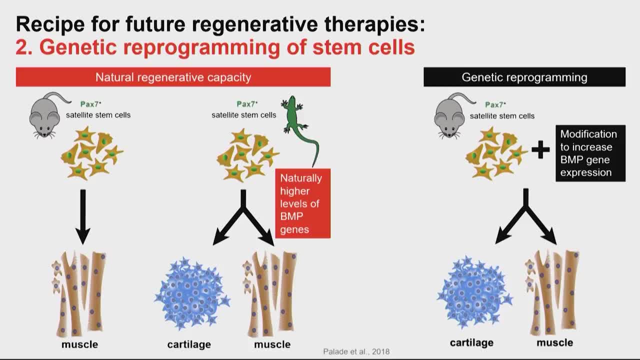 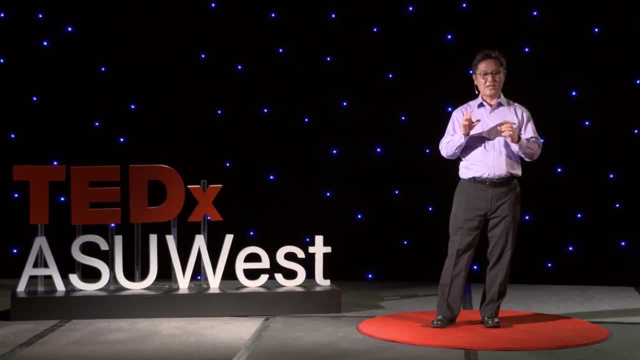 actually can then express different genes, and so it would be, need be our cells, so so they would be recognized by our body as ours. but that's within the realm of possibility, now that we're starting to get a good sense of what genes need to be on or off. now we're big animals. lizards are. 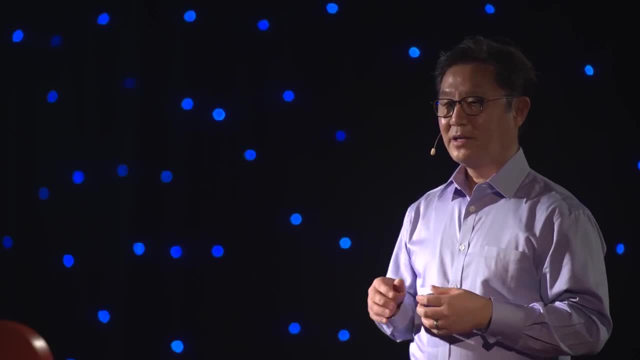 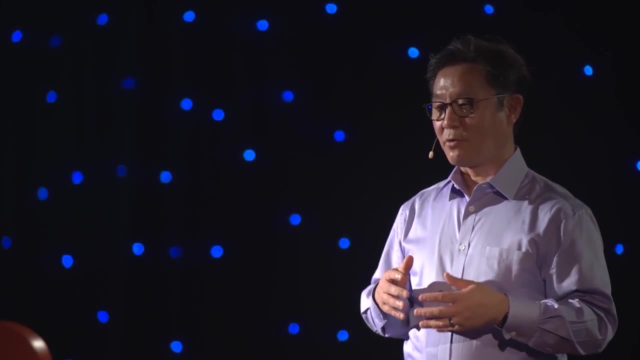 really small. you know, alligators, which we've studied, are bigger, but you know if we're replace an entire leg or arm, that's not very easy. so we're not only going to need genetic reprogram stem cells, but we're also going to need to take advantage of the best of bioengineering married. 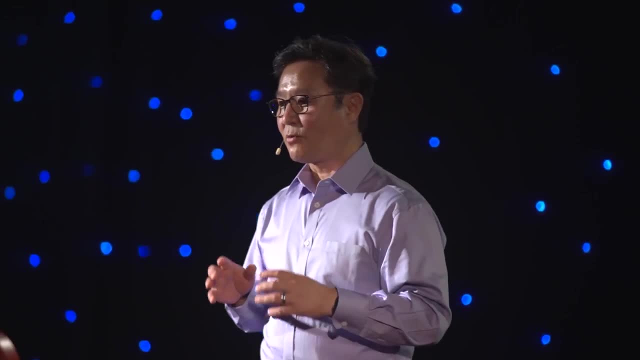 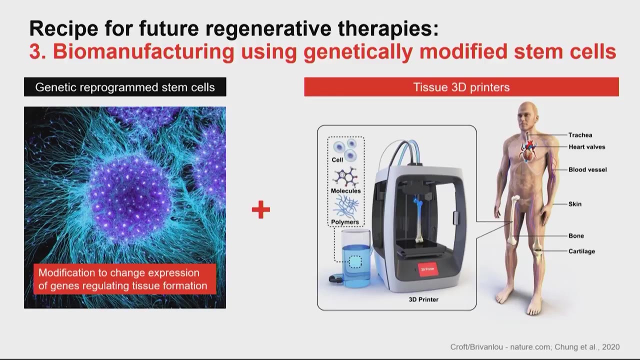 with this genetic technology. so scientists right now, and engineers are working on these 3d printers, which actually then can you combine high-tech materials and actually lay down and print, you know, tissues and cells and create structures that we couldn't create, that you know, that are just too. 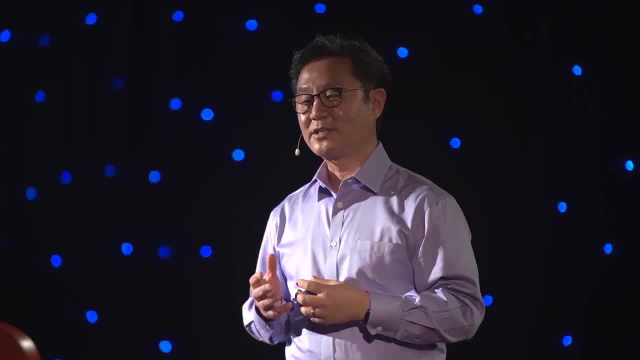 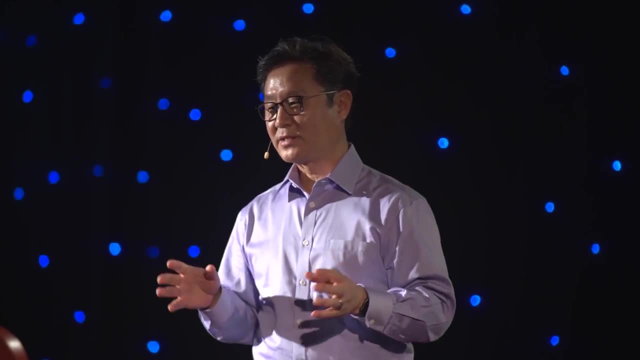 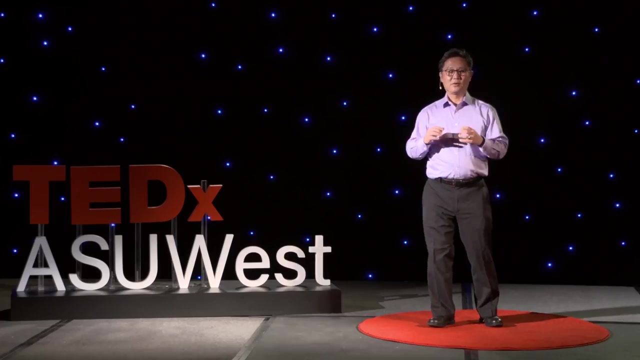 big. so, given how big we are and how big our organs are, it's likely that we're going to have to marry engineering technologies plus these sort of genetically programmed, reprogrammed cells in order to make the structures that we're going to need to replace. so that's the third part. so you know these are. 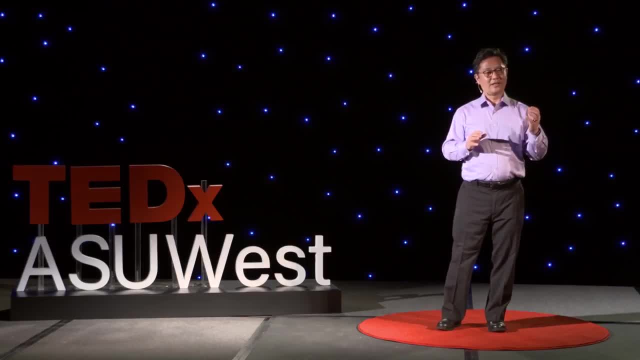 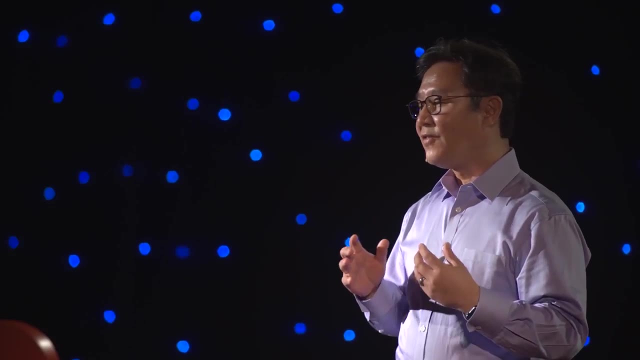 three pieces that we already see that are going to be important, you know. the first is, you know, understanding, like, what are we capable of doing in terms of regeneration, you know, and the genes involved. the second is the- the need to actually reprogram these cells. and the third is: you know something that's still very much in works. 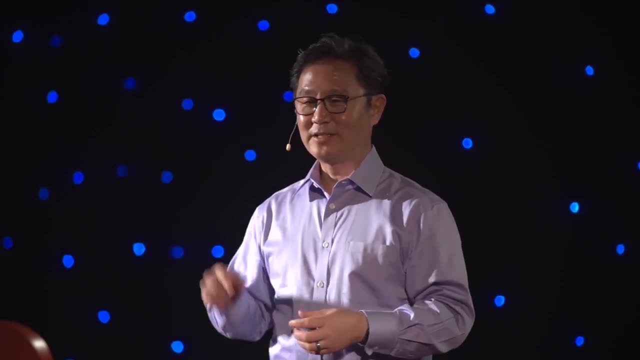 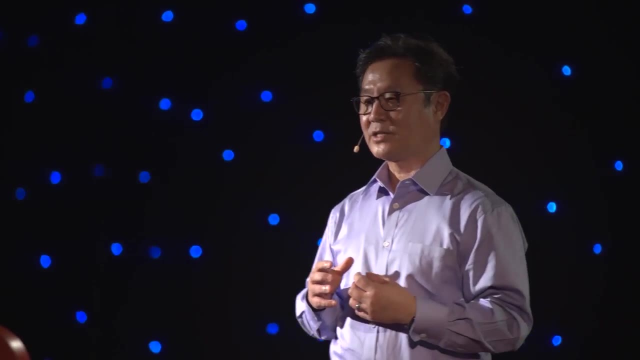 it might take decades to perfect. you know, after all, you can't just hit a button and 3D print a limb right. so this might, you know, be the work of many decades of activation to be carefully creating the right structures. but why do we need this to work? well, we are have so many critical organs that we're 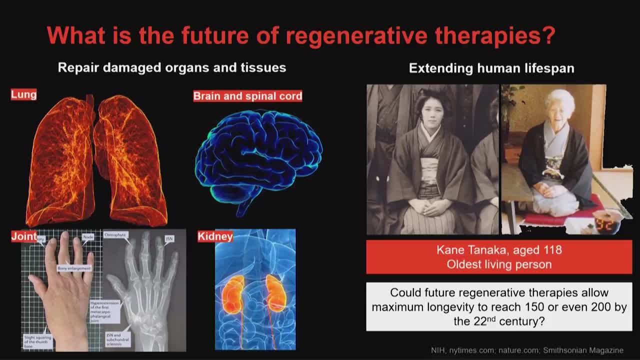 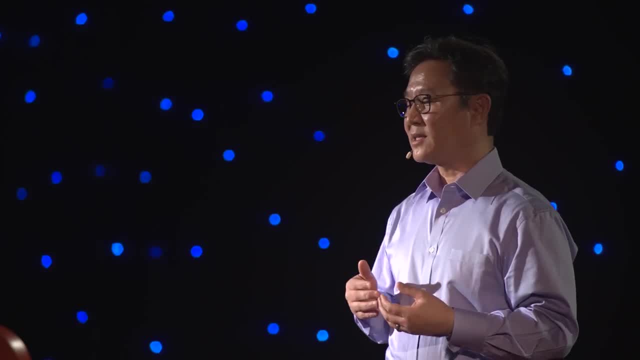 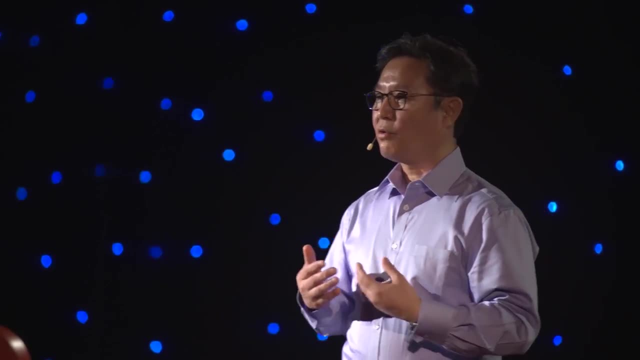 not able to regenerate. our lungs, our brain and spinal cord, our kidneys- I mean most of our organs- are damaged and you know this has led to tremendous suffering and illness. you know, and many of you may have family members or people you know that are really suffering because you know their organs. 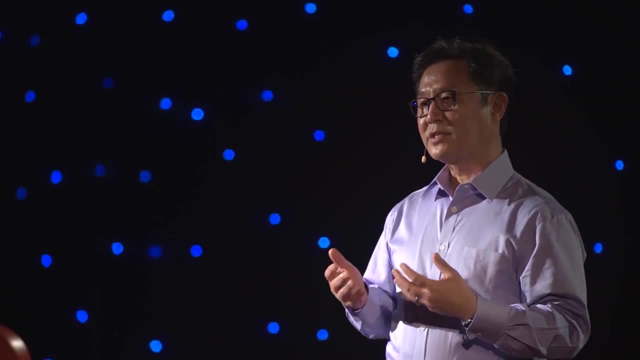 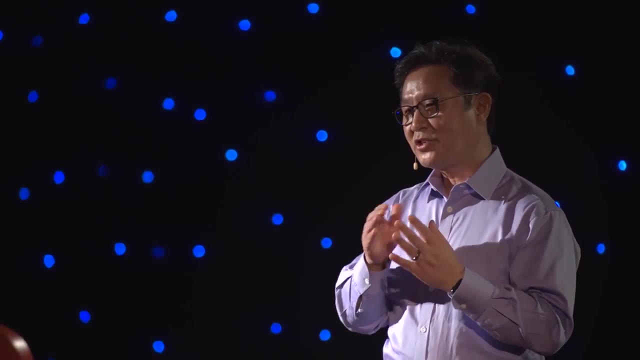 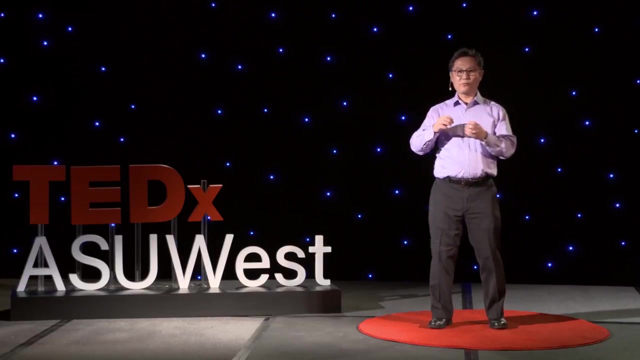 have failed or organs are damaged also, even more simply, so to speak. you know, you probably know a lot of people that have arthritis or osteoarthritis, and the, the tissue that's in the joints is relatively simple, it's articular cartilage, and the lizards, when they regrow their tails, they grow lots. 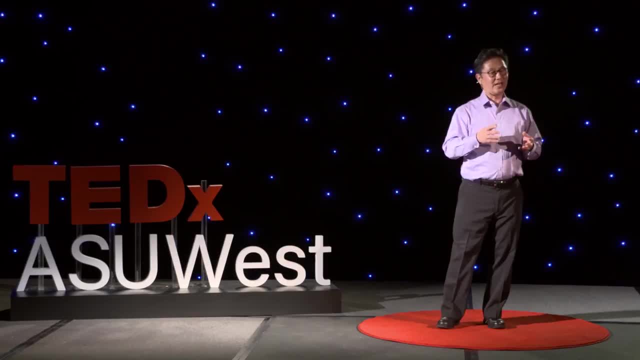 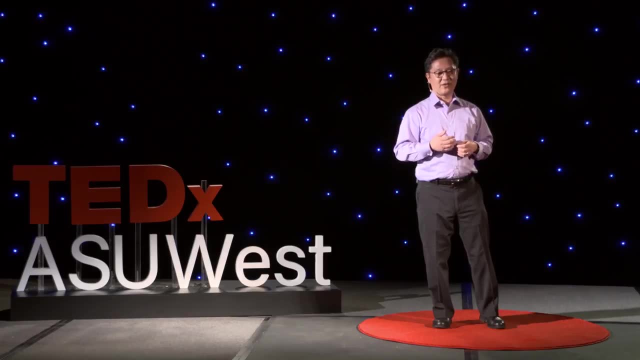 of that. I mean, they can just do that really easily. so, even you know, understanding well, how are the lizards able to regrow this cartilage? that would, just, you know, make our joints work so much better, would be a huge advance. and of course, you know, 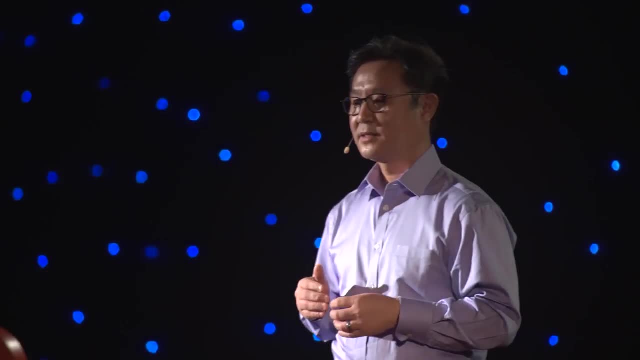 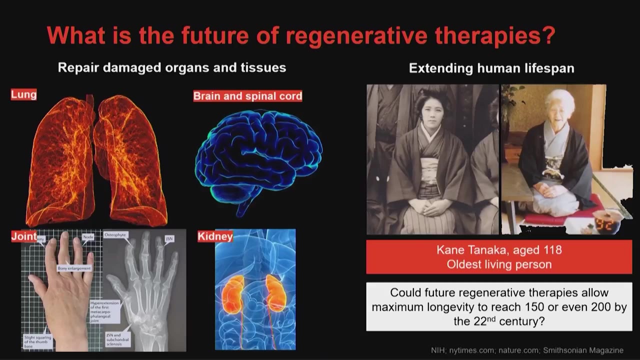 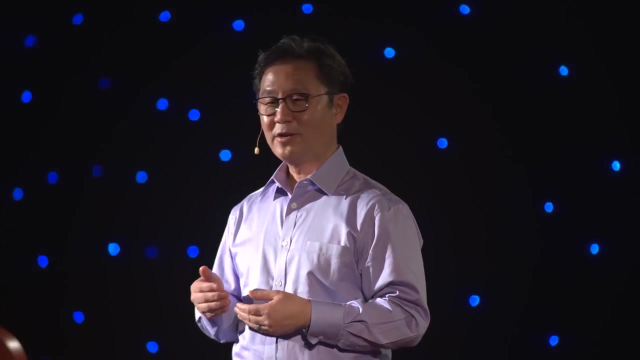 you know, we, you know, as humans, have limited lifespans. so the oldest human being alive right now is Kanetanaka and she is 118 years old, and that's old, but I think there are people, probably in this audience right now, that would like to live to 150 or 200, and we're not going to get. 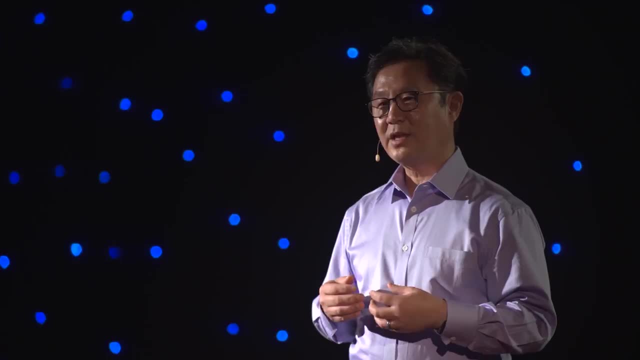 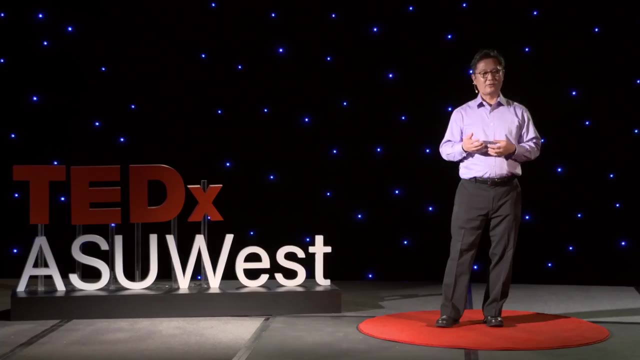 there, naturally right. so how do we do that? well, we know that our organs wear out. they're not going to last that long, but if we're able to replace them, if we're able to repair damaged brain tissue or, you know, damaged heart tissue, then we actually could potentially extend our lifespan. so you know,